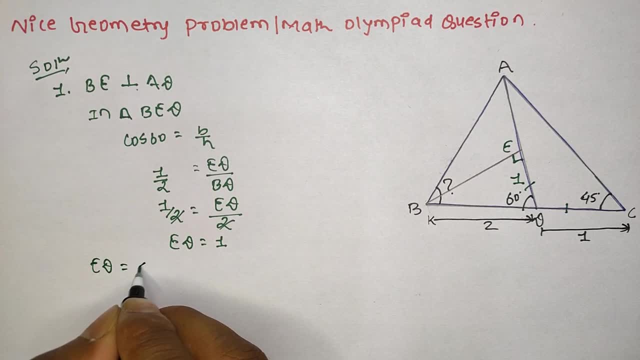 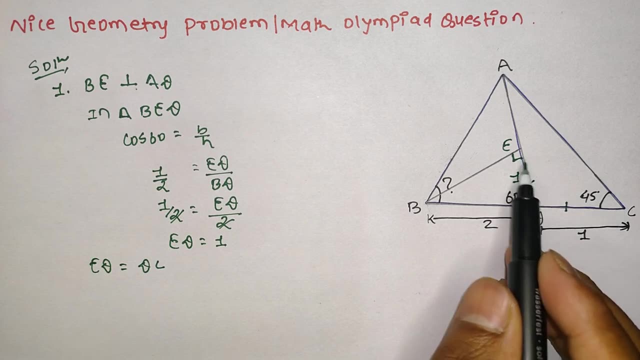 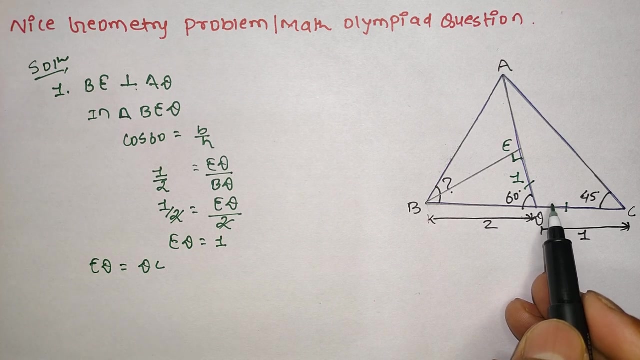 here our ED is equals to DC, which is equal to each other, then these two side are equal. we can draw a line here, ENC, such that we can make a triangle, DEC, and so that DC is also an isosceles triangle. okay, by this way. so here you. 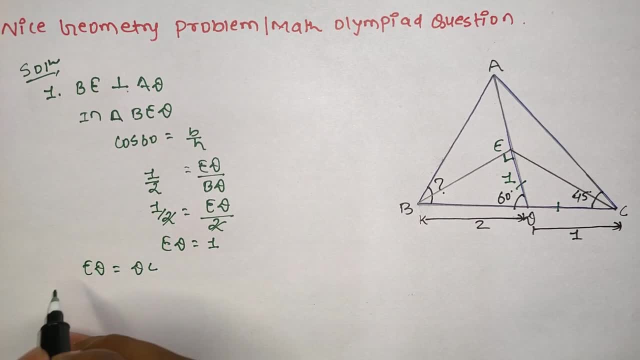 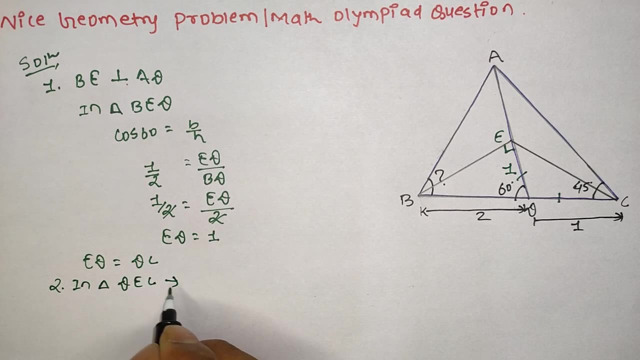 can see that we have a triangle DEC. we can going to look in second step in triangle DEC and you can say that DEC is an isosceles triangle because the two length, the two length of this triangle, that is, and DC, are equal to each other. so here this angle and this angle we can draw. 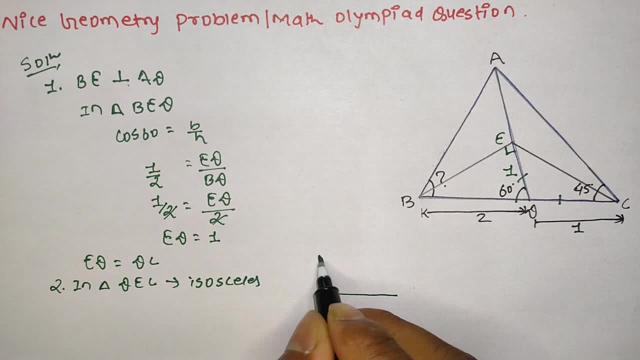 a line, draw a triangle here. this is our triangle, this is our C, this is our D and this is our A. so here, this side and this side are equal. it means that the opposite angle of this side is this one and the opposite angle of the side is: 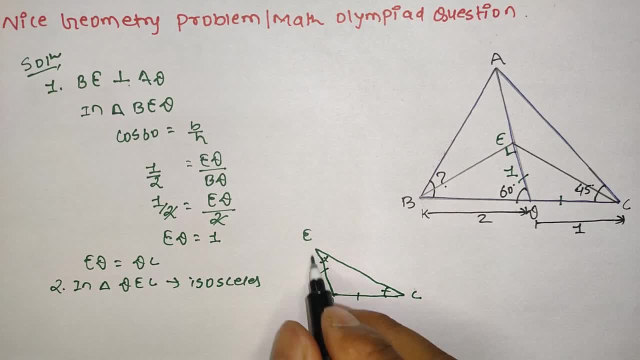 this one. these two angles are equal to each other and in this triangle we are using a extra angle theorem. so, according to extra-angle, our this angle is our exterior angle. that is this 60 degree. okay, so 60 degree is an exterior angle which is equal to the sum of two opposite interior angle. 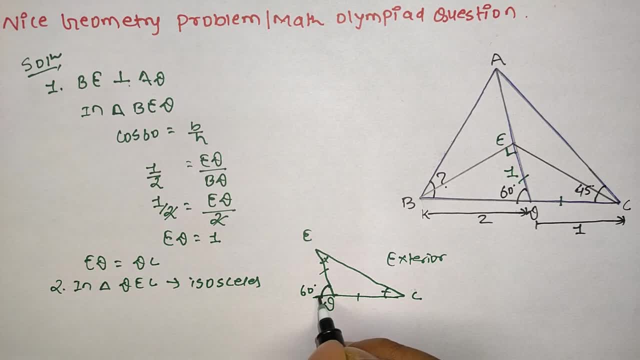 so this one and this one, the sum of these two angle must be equal to 60 degree and as you know that these two are equal. so if I assume the same as X, then X plus X is equal to 60 degree. so we can get the value of X is equal to 30. 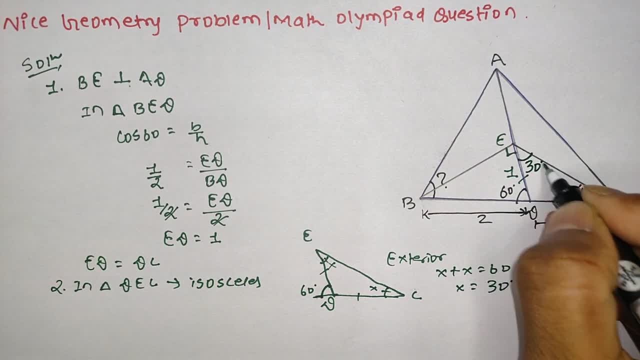 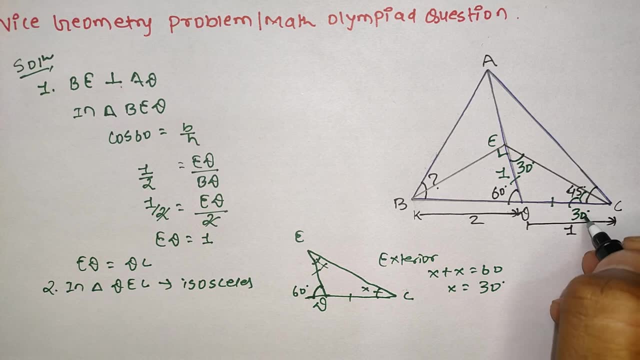 degree. so our this angle is our 30 degree. similarly, our this angle is also 30 degree, isn't it? and as you know that our this angle is 30 degree, and here in triangle, PED, this is our 90 degree, this is our 60 degree. then you can also say: 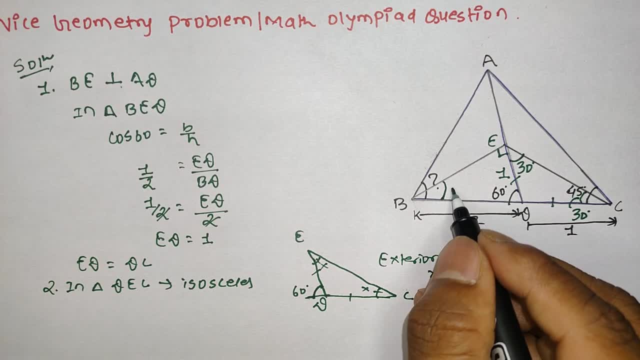 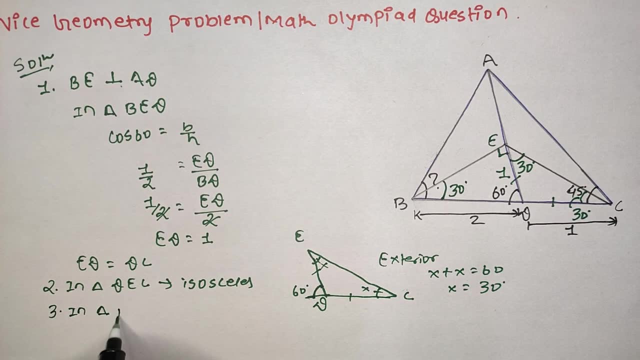 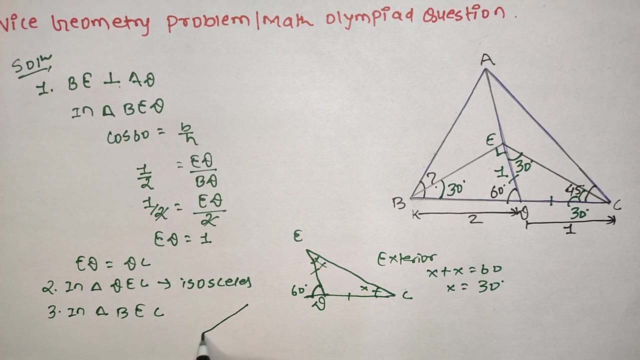 that 90 plus 60, it is 150 and remaining this angle is 30 degree. then in third step, we can look in triangle BEC. so here in triangle BEC, you can see that we have a triangle like this way: okay, this is our A, this is our B and this is our C. this angle is our 30. 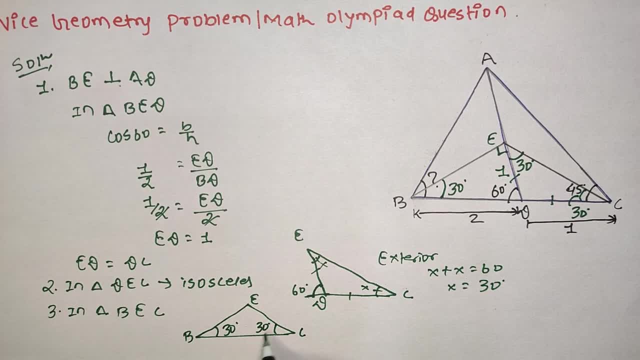 degree, and this is also our 30 degree. so if these two angles are equal, then the opposite angle of sorry, the opposite side of this angle, is this one and the opposite of this angle is this one. both are equal to each other. that is, these two side lanes are equal to each other, isn't it? 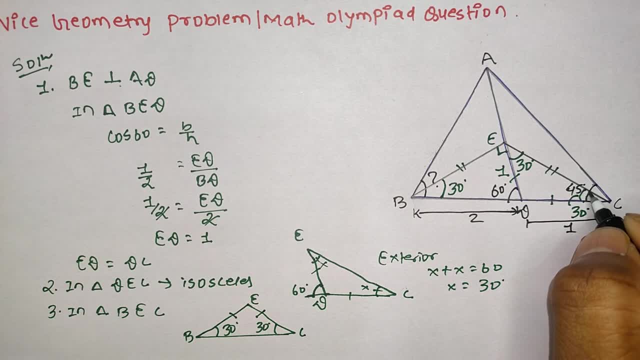 we have this whole angle is 45 degree and this only angle below angle is 30 degree. then you can clearly say that this is our 15 degree. that is 45 minus 30. so this is our 15 degree. then in fourth step we are going to look on the 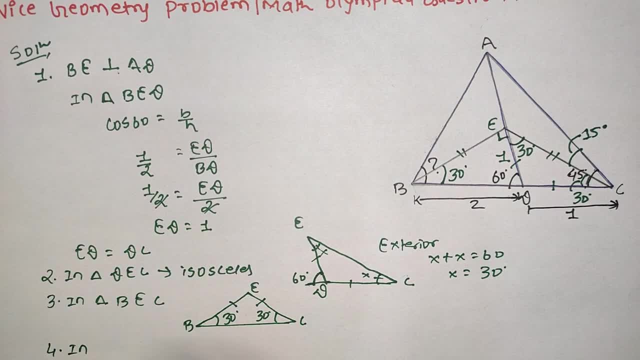 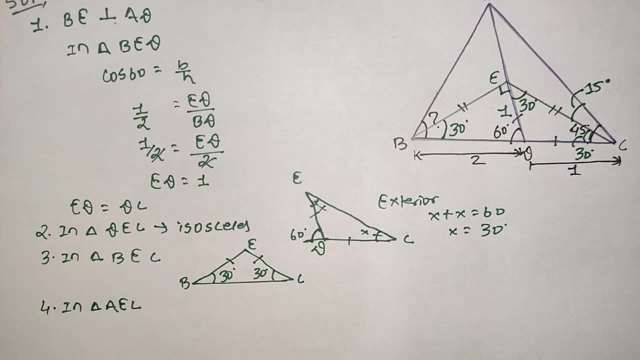 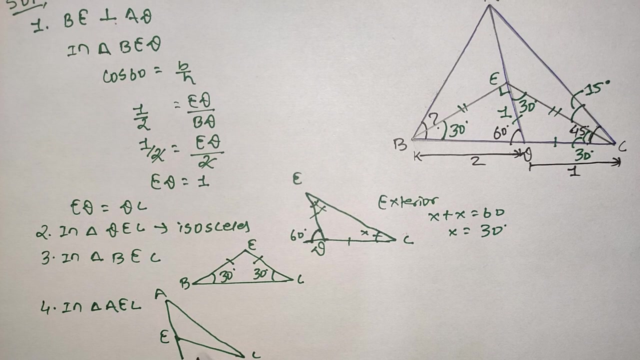 triangle, our AEC. okay, so in triangle, AEC. so here we have a triangle like this way you can draw. here we have a triangle like this way: this is our C, this is our A, and this is our A, and we can extend this line and again we can use our X-triangle theorem in this triangle. so here we have this. 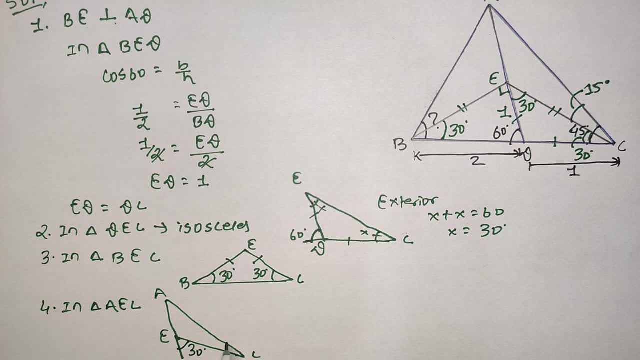 angle, that is, this one is our 30 degree, and this is already we have found here. that is 15 degree. then this is the X-triangle, which is equal to the sum of two opposite inter angle. that is this angle. it equals to the sum of this angle plus this one. so you 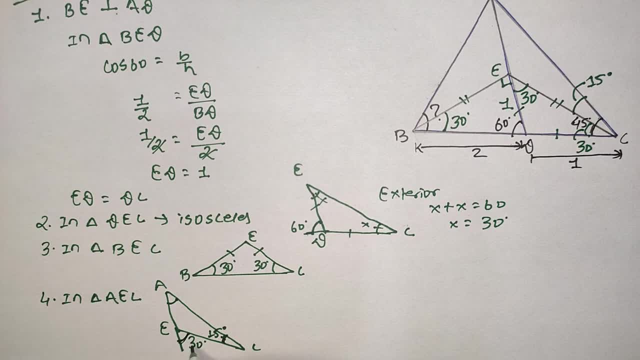 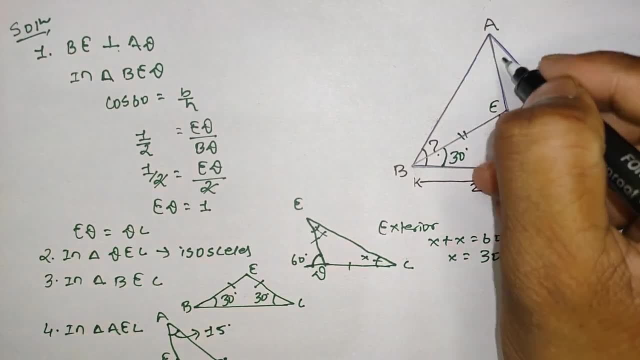 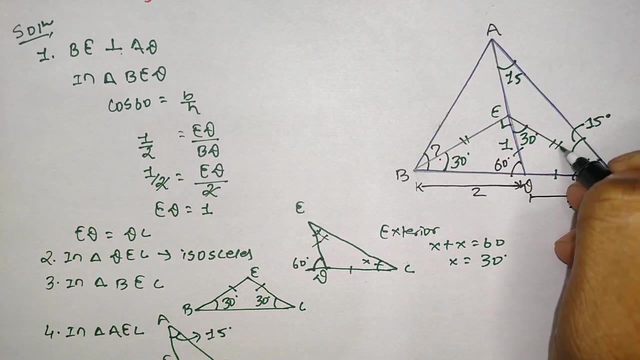 this is 15 degree. so to make the sum of this angle plus this angle 30, this angle must be equals to 15 degree, isn't it? so this angle, that is, our, this angle, is 15 degree. so this is 15 degree and this is 15 degree. it means that this side length, this side length, opposite angle of this. 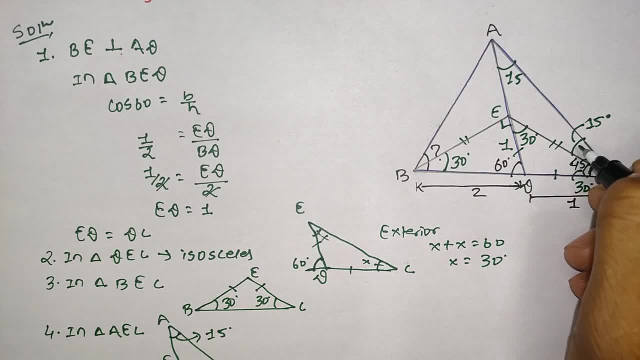 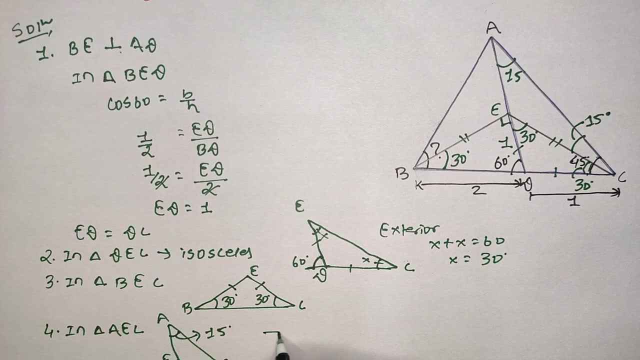 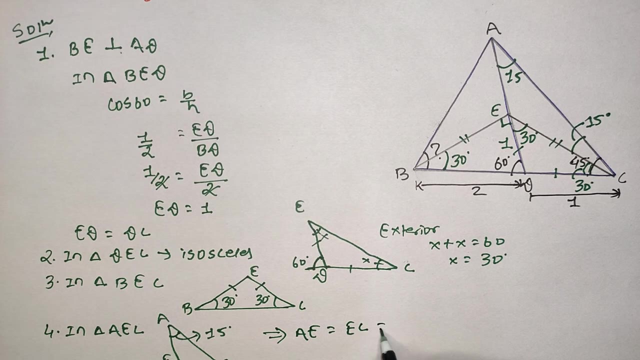 one. that is this sorry. opposite side of this angle is this one, and the other side of this angle is this one: these two length, that is, ae and ec, must be equals to each other. from here we can conclude that ae is equals to ec and ae is equals to ec, and ec is all already equals to. ec is already equals to. 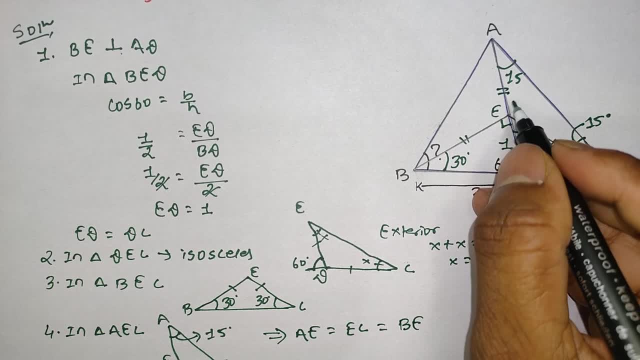 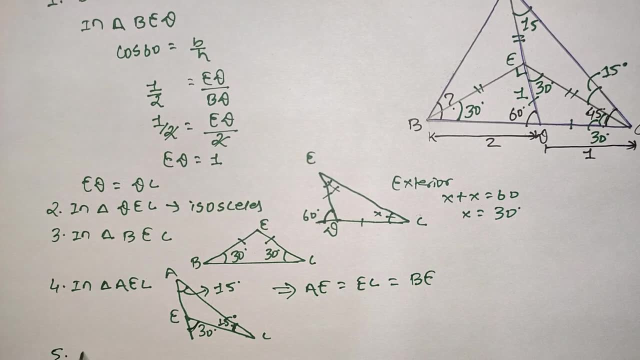 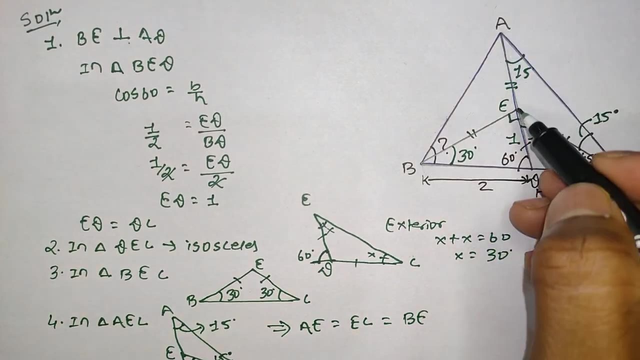 be. that is, this side length and this side length are equal to each other. this one, this one and this one are equal to each other. then in fifth step we are going to look on the triangle in triangle a b e. that is our, this triangle a e b. so here we have this side length and this side length are